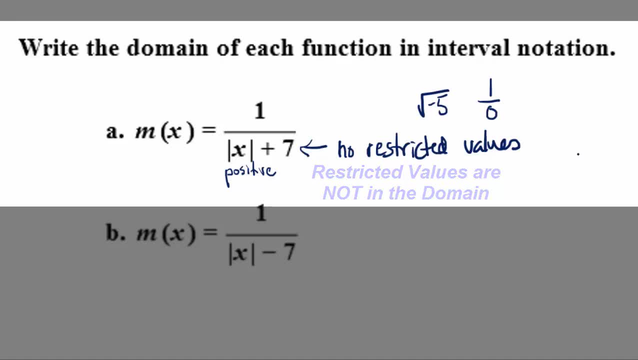 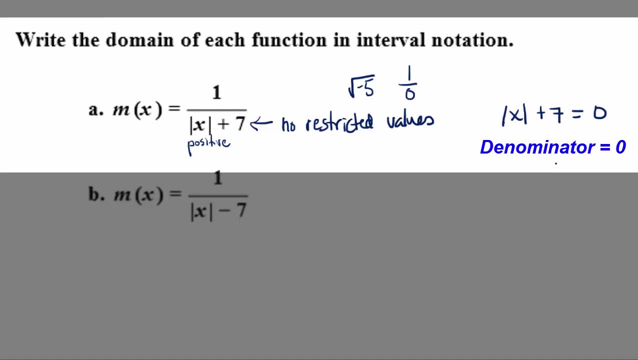 Because you're not solving an equation. So here's another way to think about it: Whenever you have a denominator, set the denominator equal to zero- In this case, absolute value of x plus seven equals zero- and then solve the resulting equation. 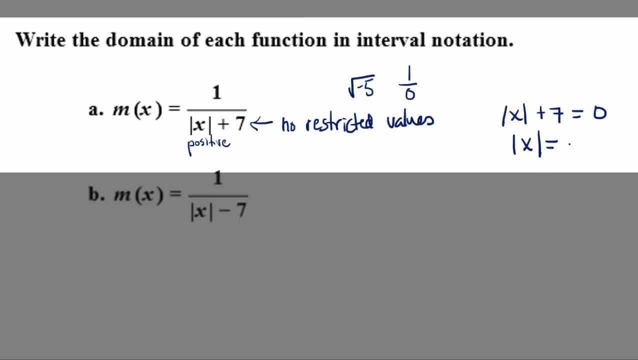 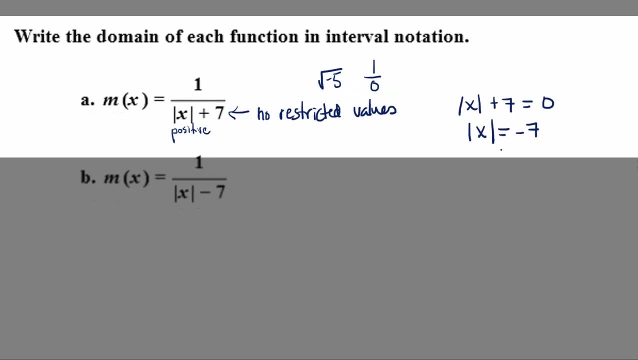 This is an absolute value equation. This would give us: the absolute value of x equals negative seven when we isolate the absolute value. So here again we see that it's not possible for this to have a solution, because the absolute value of a number is never going to be equal to a negative. No solution. 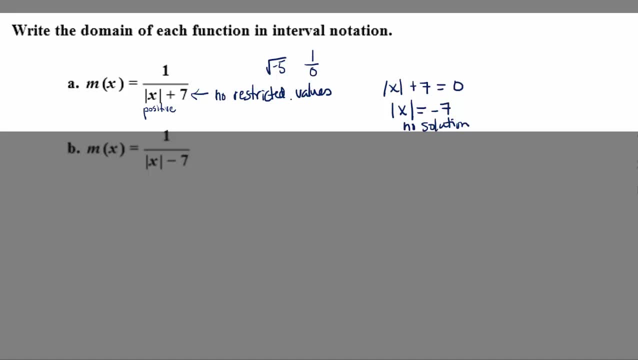 This means that this function m of x has no restricted values, or in other words, that the domain includes everything Negative, infinity to infinity, All real numbers. Now, there are several ways to represent this, but in the instructions we were asked for interval notation. 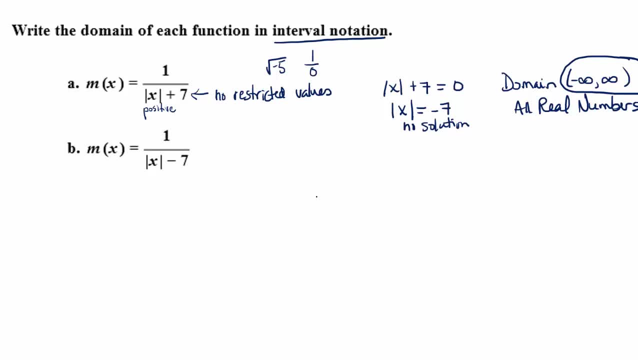 So the appropriate response would be negative. infinity to infinity. That's the solution to part a. Part b is a very similar function. Again, the only thing that can go wrong is if we were to plug in a number that would cause the denominator to equal zero. 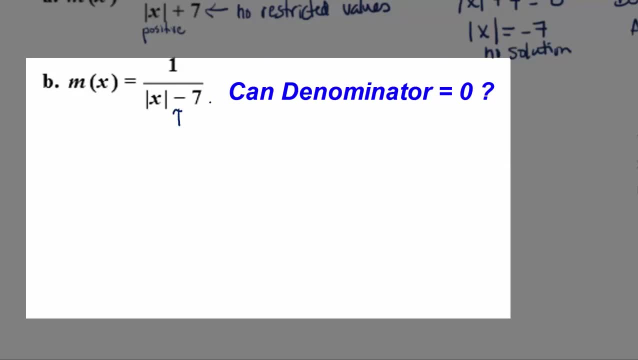 Now, in this case we're subtracting. So when we subtract two positive numbers, it is possible to get zero. So let's go ahead and set up the equation that we solve when we want to find out if there are any restricted values for a rational expression. 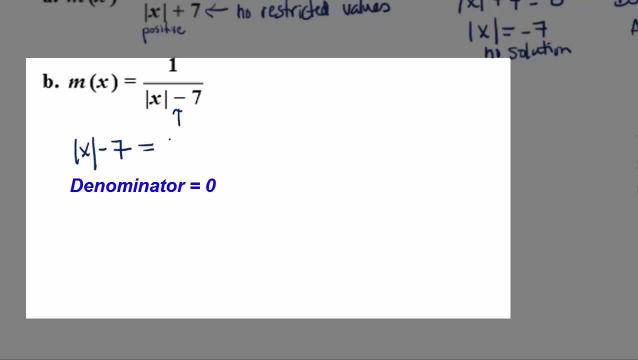 Absolute value of x minus seven is the denominator. I'm going to set that equal to zero and solve for x. Isolating the absolute value, we get absolute value of x equals positive seven, which is possible. In fact, If the absolute value of x is equal to positive 7, there are two possibilities. 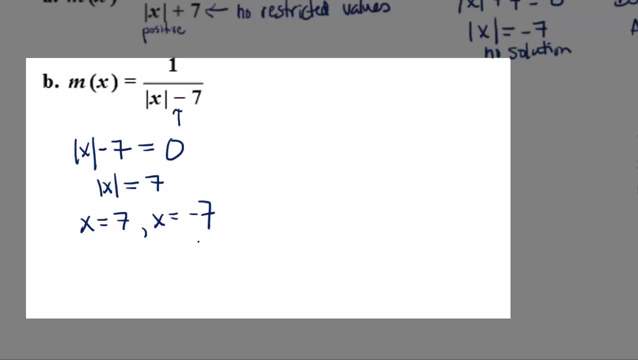 Either x is 7 or x is negative 7.. Well, that makes sense, right? If we were to plug 7 or negative 7 into this denominator, we would get 7 minus 7 equals 0. So is the domain 7 and negative 7?. 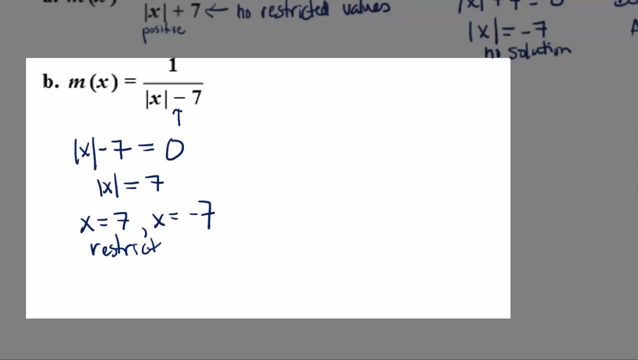 No, these are the restricted values, the ones we're not allowed to plug in. So the domain is going to include everything but those values. Since we're going to write our answer in interval notation, I find using a number line is really helpful. 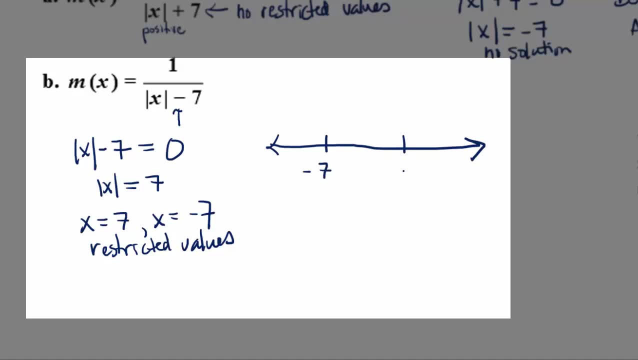 What I'm going to do is I'm going to mark off the restricted values- negative 7 and 7, in their proper numerical order. I'm going to cross them off because these are the numbers that we don't want. What we do want is everything in between.